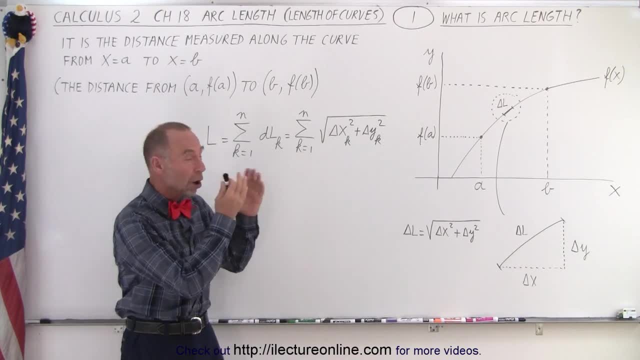 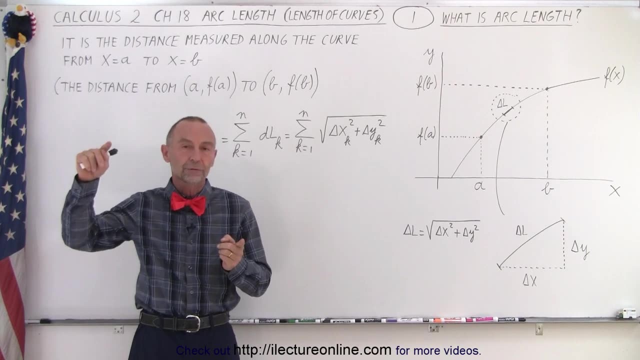 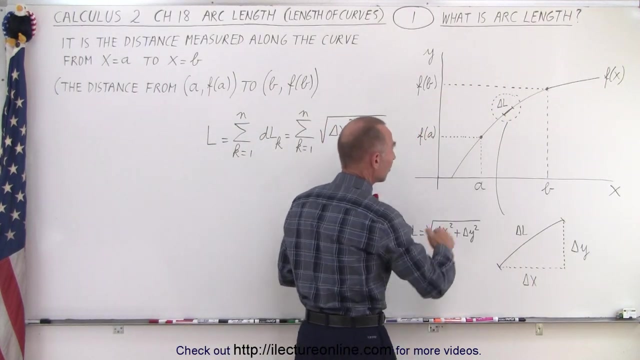 really good idea to add a section on what we call arc length. Now, arc length, well, what is it? It's the measure of length along a curve, from one point on the curve to another point on the curve. So, mathematically, if you want to draw it out on an xy graph, you can see that here is a curve. 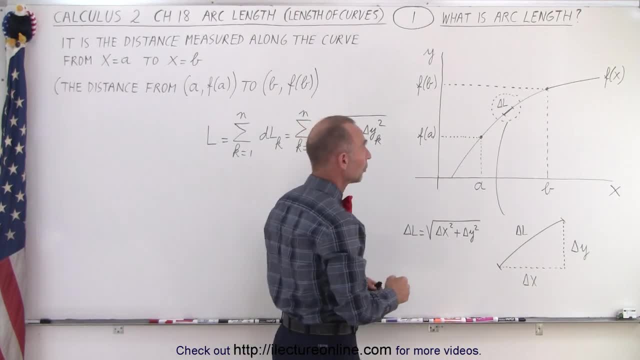 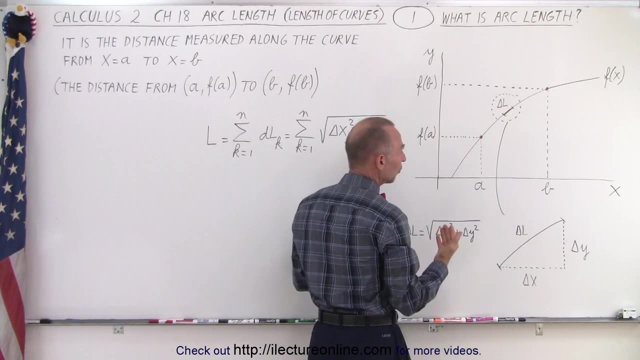 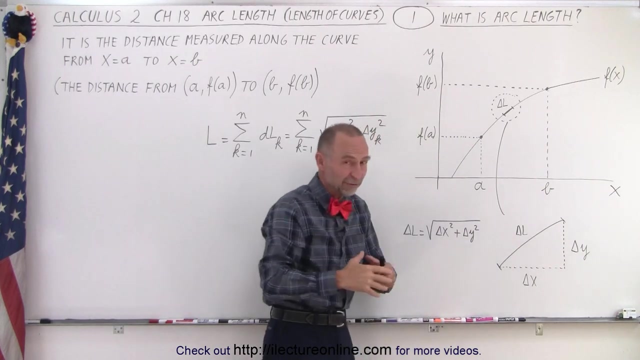 let's say that it's a function of x and you want to know the distance from this point to this point on the curve, so you try to measure it along that curve. Now notice, typically they'll have the limits in terms of the x values: from x equals a to x equals b. They don't always say: 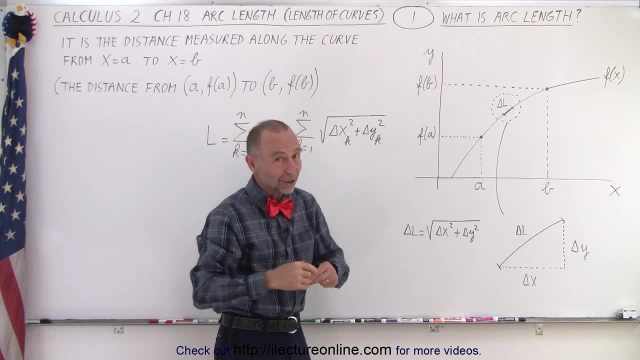 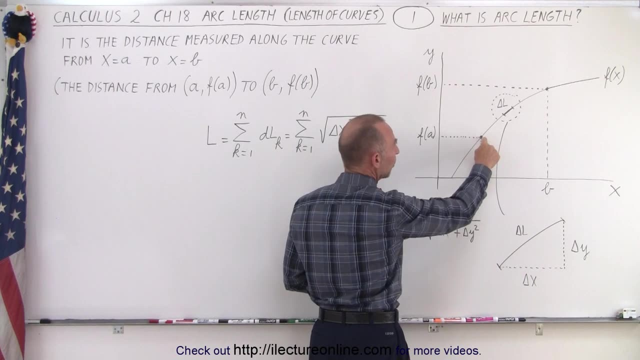 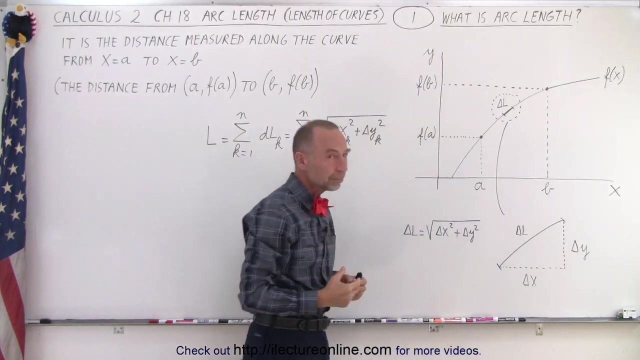 from x equals a to x equals b. they just say from a to b and you have to realize they really meant from x equals a to x equals b. Sometimes they will actually give you the point, both the x and the y coordinate of the point 1, and the x and the y coordinate of the point 2.. So essentially, 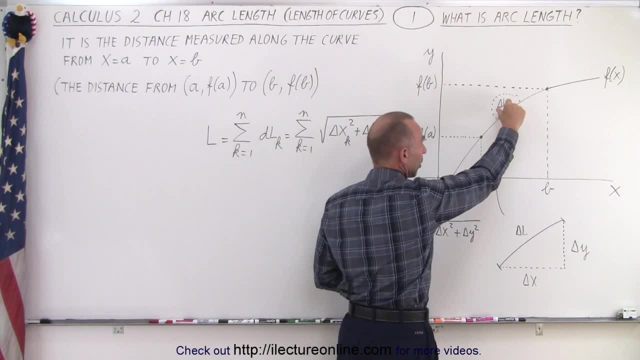 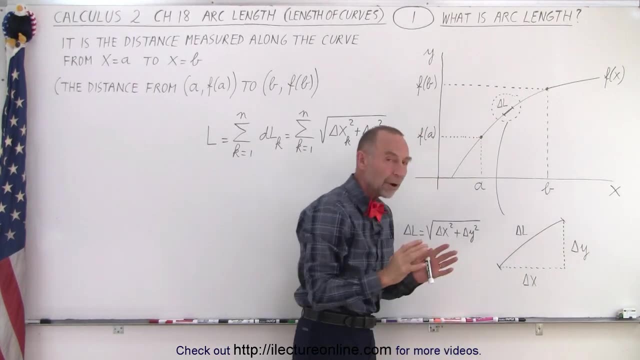 what we do, then is we snip it up into small little sections, small little delta l's, and notice that if you blow this up, you can see that the delta l, even though it's curved, you can approximate the length by using Pythagorean theorem. We can say that delta l is equal to the square root of the. 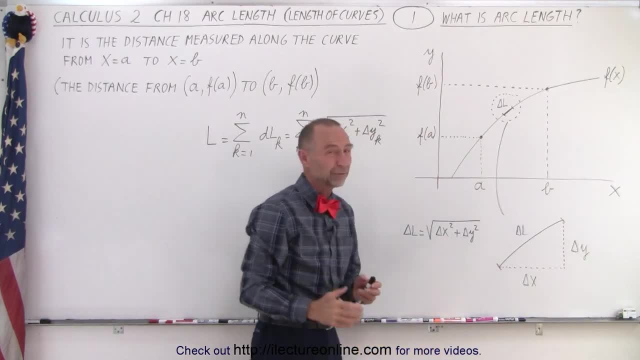 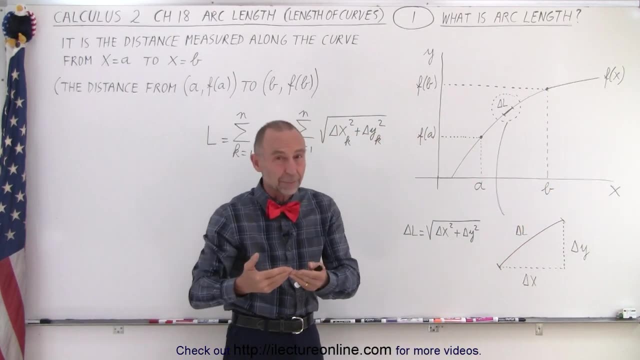 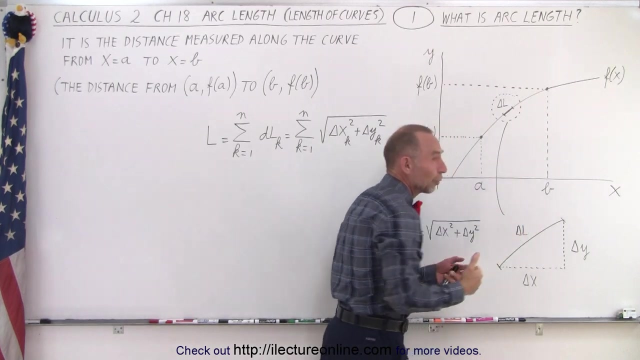 change in x squared plus the change in y squared. Now, of course, for that to be actually true, we need to shrink the size of delta l until it, essentially in the limit, goes to zero. Well then, in the limit we'll have an infinite number of little delta l's. we add them all up and of. 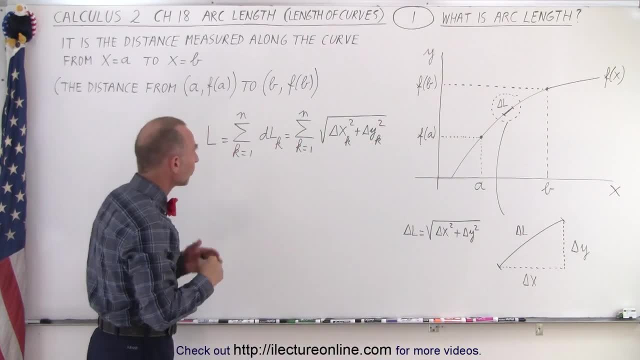 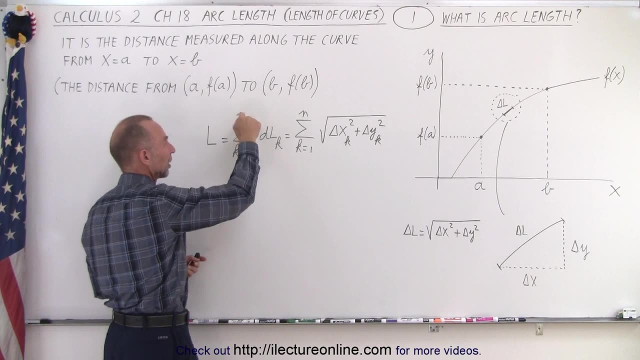 course that sounds like integration, But we want to first take a look at it this way: We want to say that the length of the curve is the length of the curve, and we want to say that the length of the curve is equal to the sum of all the little sections, however many sections there are. Let's 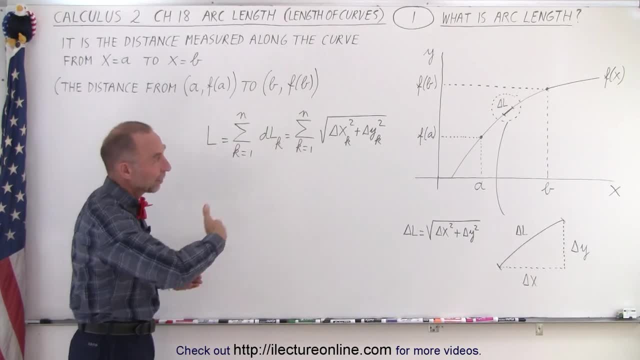 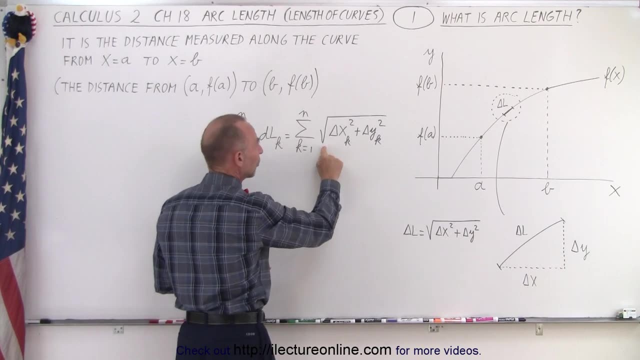 say there's n number of sections, Of course, when n goes to infinity, that's when you have an integration, that's when you get the exact length of that curve. So we can simply say it's the sum of all the square roots of delta x squared plus delta y squared from k, equals 1 to n, and then 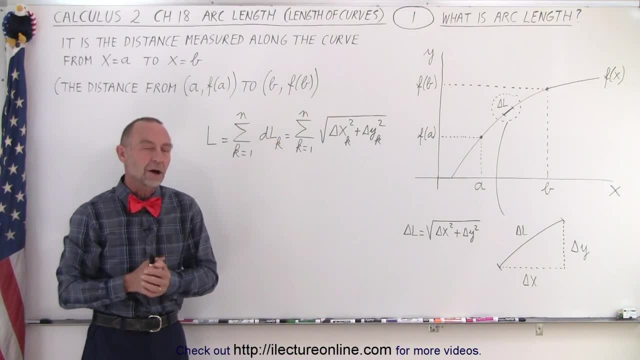 of course, in the end going to infinity. So that's the concept of the arc length. We can also call it the length of the curve. Now, what you're going to do is you're going to take the length of the curve and you're going to